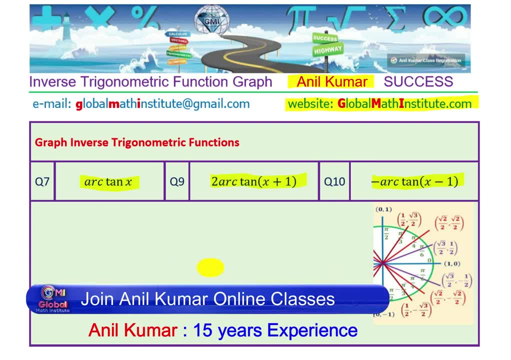 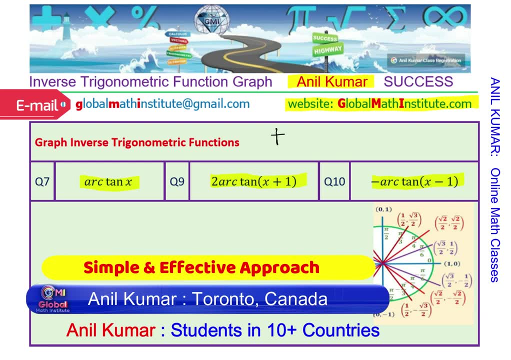 is also a function. So let us begin with the basic characteristics of tan x, So we will first understand what is tan x. So t is small, so tan x, That means y equals to tan x. So, as you know, the graph of tan inverse x is periodic, with a period of pi right, not 2 pi. 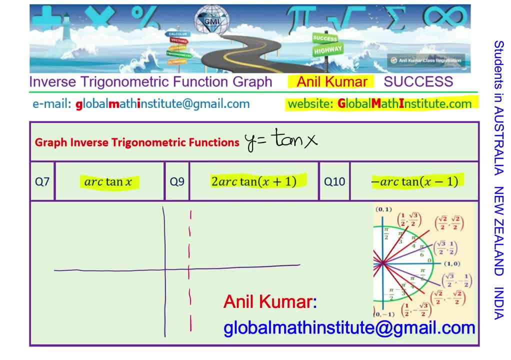 So we have vertical asymptotes at every pi by 2, alternate or multiples of pi by 2.. So what I am showing you here are the vertical asymptotes at minus pi by 2 and at pi by 2, correct, So this is a period of pi. 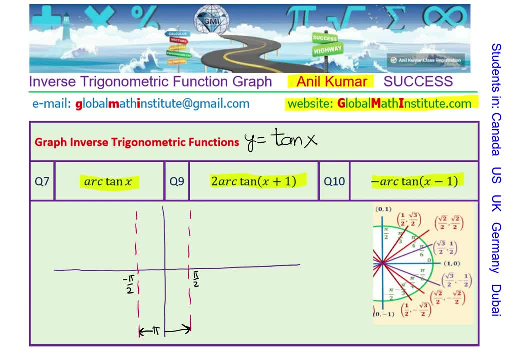 Which we are talking about. As you know, the function really repeats, And so at every odd multiple of pi by 2, we are going to have a vertical asymptote, right? So if you add pi to this, this will be 3 pi by 2.. 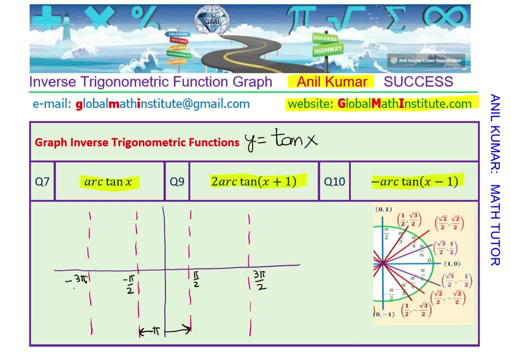 You get the idea. And minus 3, pi by 2.. So first we are going to sketch the graph of tan function, which clearly is kind of like this. So we are going to sketch the graph of tan function, which clearly is kind of like this: 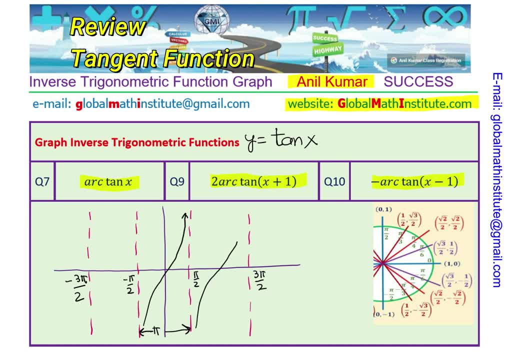 So we are going to sketch the graph of tan function, which clearly is kind of like this, Which clearly is kind of like this: So that is always increasing in its particular interval of pi within the 2 vertical asymptotes, correct? So that is the graph. 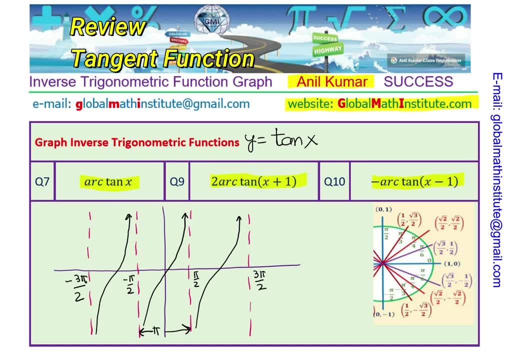 So whenever you sketch a graph, you need 5 critical things to work on. So what are the five things here? Two horizontal asymptotes and going through the origin- and this point is very critical- which is, you know, it has at 5 what. 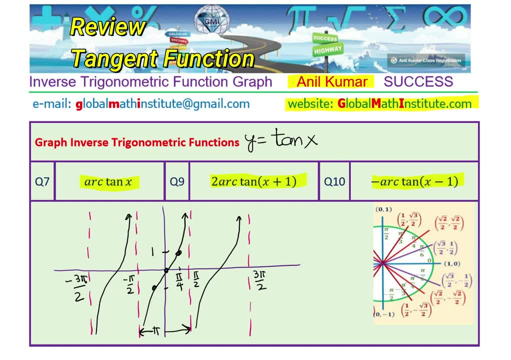 at pi by 4, value of 1, and even at minus pi by 4, we have minus 1.. As you know, tangent is an odd function, so you can see the symmetry about the origin. So, since it fails the horizontal line test, we do a restriction. so we are going to restrict, right. So the restriction here is: 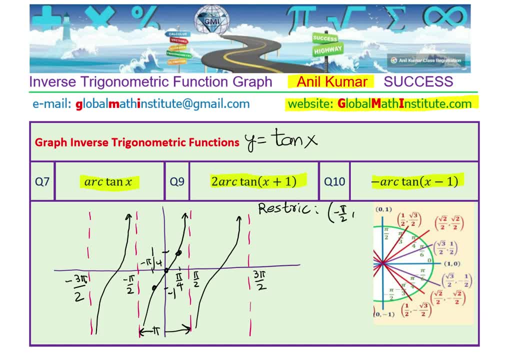 from minus pi by 2 to plus pi by 2. is that clear to you? So now we are working in this particular domain, which is from minus pi by 2 to pi by 2.. So the domain is restricted. we will also call this as our domain right Now, within this domain, what is the range? 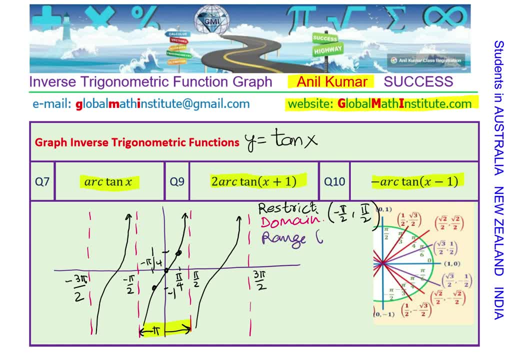 As you can see, ranges from minus infinity to infinity, and the critical points which we are considering are: at minus pi by 4, we have a value minus 1. at 0: 0, we have 0, 0, and at pi by 4, we have 1.. 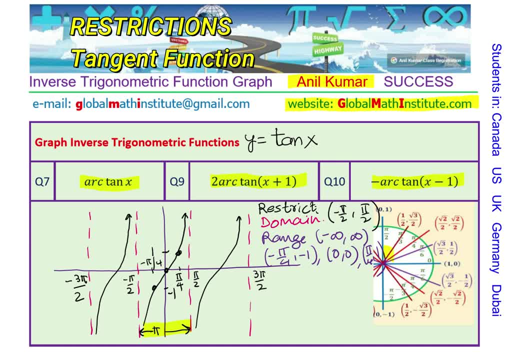 You will also notice that here I have sketched a unit circle in quadrant 1 and quadrant 4 is for a reason. Reason is that we have restricted our tangent function in quadrant 1 and 4 minus pi by 2 to pi by 2, right? So this is minus pi by 2, and then from here to here we have pi by. 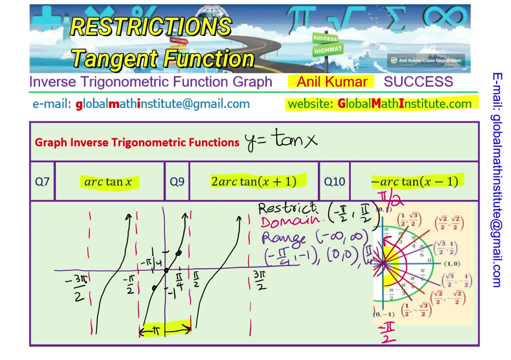 2 make sense, correct. So we will be only considering these two quadrants on the right, to look into the values of inverse tan x. perfect, So I hope you got the concept. So we have our base basic parent function, which is tan x, and from here we are going to now sketch arc tan x. 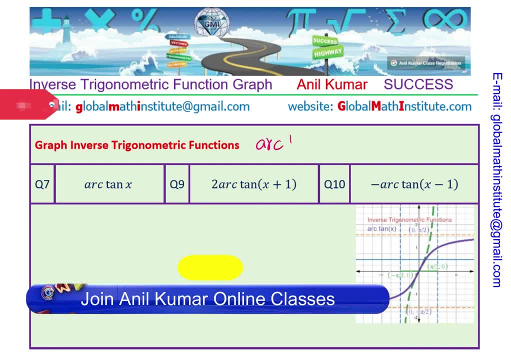 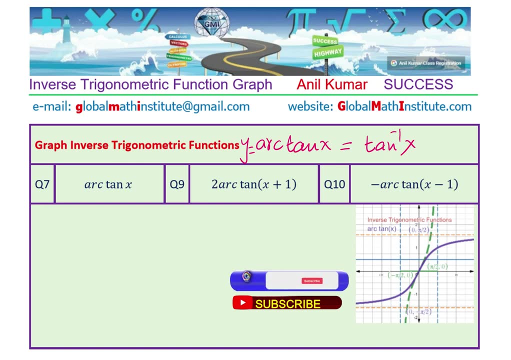 So let us now begin with arc tan x, also written as tan inverse x, correct? So of course, this is equal to y, right? So that is what? So now, what we are doing here is, let us summarize that, as far as the tan, 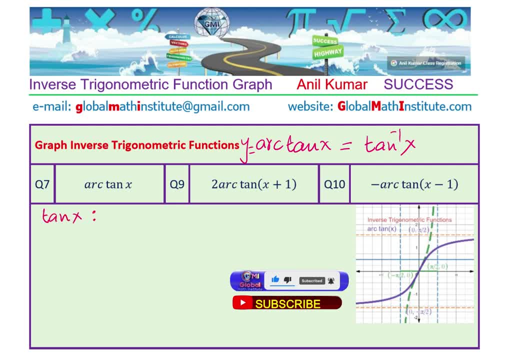 x is concerned. in that case we have critical points. as minus pi by 4, we have a value minus 1. at origin it is 0, 0, and then at pi by 4 we have the point which is at 1 plus we have vertical asymptotes. at x equals to minus pi by 2 and pi by 2, very good. 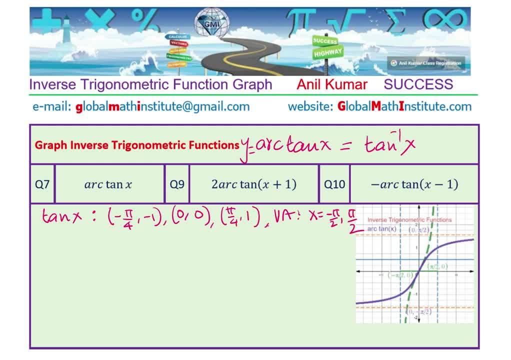 So that is about tan x. Now when you do inverse of this, you get y equals to arc tan x. So when you do arc tan x, x and y points swap, So these points now become minus 1, minus pi by 4. make sense right. 0, 0, perfect 1 pi by 4. 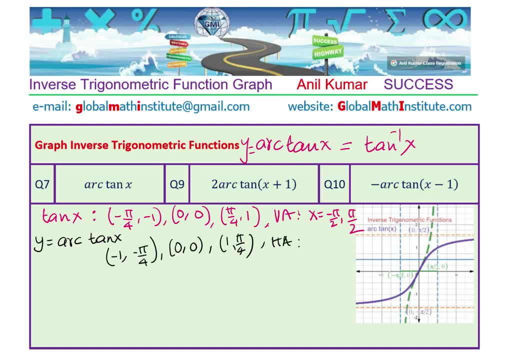 and vertical asymptotes become horizontal asymptotes, which will be now y equal to minus, pi by 2 to pi by 2.. Makes sense, correct? So that is how the points get changed. You see the domain and range also swaps. Now the domain is all real numbers and the range is restricted between minus. 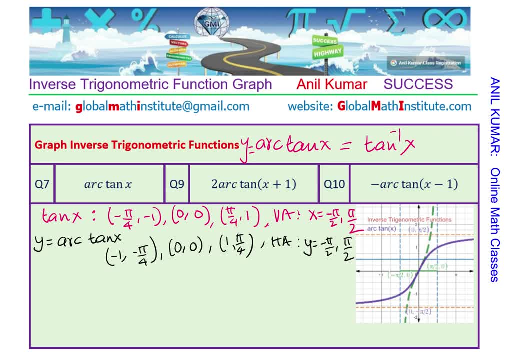 pi by 2 to pi by 2.. So let's sketch it. now It's time to sketch. Very simple, correct? So we are drawing this line: y equals to x, correct, And a vertical line here indicating y. right Now. 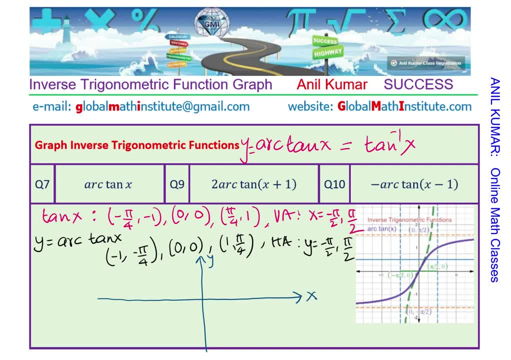 x and y coordinates correct, So we will do the horizontal asymptotes which are for us pi by 2 and minus pi by 2.. Scale is not there right, So it's not to this key And the three critical points which are going through the origin. 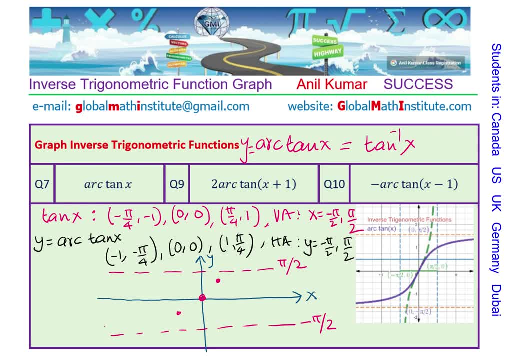 symmetrically placed right. Do you see that? So joining them horizontal asymptotes at pi by 2 and minus pi by 2, we have our tan graph- Makes sense where this particular point is now at 1. pi by 4, right, This is of course at origin, and here we have: at minus 1, we have the 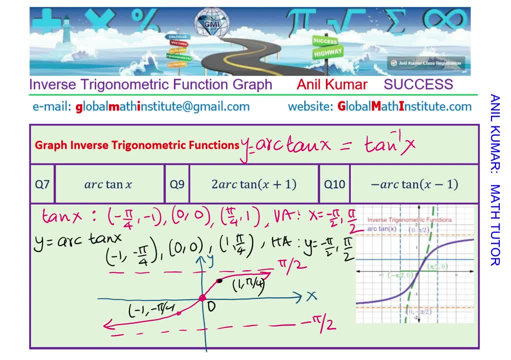 value as minus pi by 4, correct. So this is minus 1 and that is minus pi by 4.. Makes sense. So the gradient has those radian pi by 4, pi by 2 and all those things. You get the idea right. So the 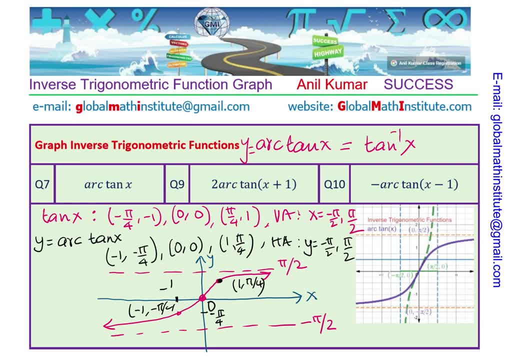 earlier we had that radian values of along the x axis. Now they are along the y axis, right, And 1,, 2,, 3,, 4, these numbers are written on the x axis. Makes sense? This is 1 for you, correct? So? 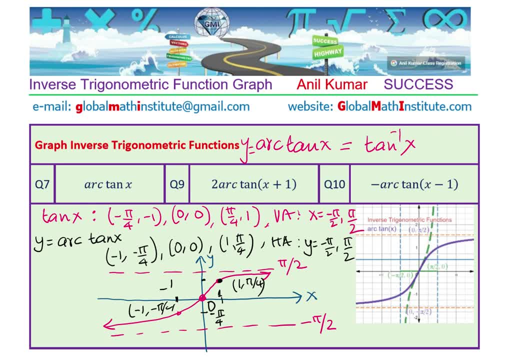 1 minus 1 in this. and here we know we will write this as half of pi by 2, which is pi by 4.. Makes sense? That becomes your graph. So this is 1 minus 1, right, So this is 1 minus 1, right? So this is. 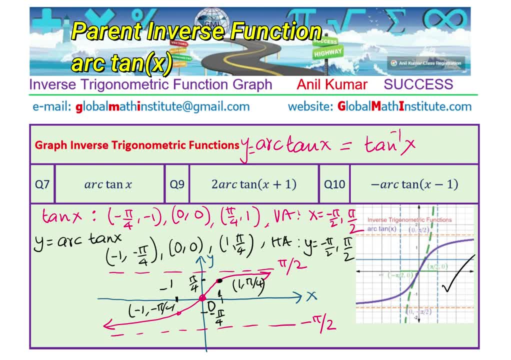 1 minus 1, right, So this is 1 minus 1.. Now the last one. this graph, exact graph from the graphing calculator, has been shown on the right. Now the whole idea here is: once you understand this particular R-tan graph, we can actually sketch the transformed functions right. So simple. 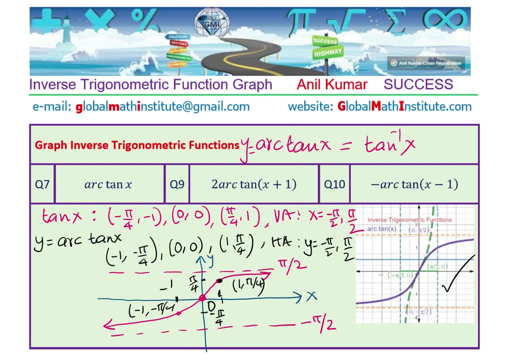 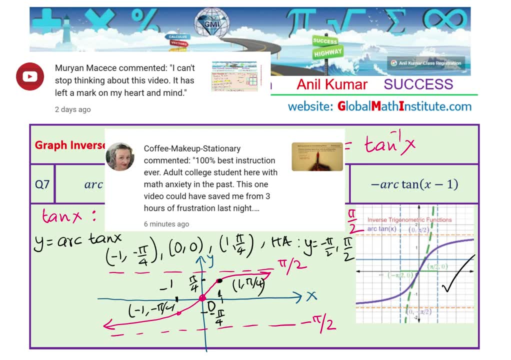 as that, I hope the concepts are absolutely clear. While feel free to write your comment, Share your views. Let me also thank all the viewers and subscribers who are really watching our videos, posting excellent comments and citations. Thank you very much. 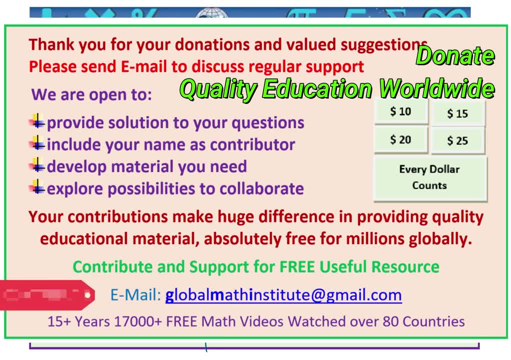 sessions, and special thanks to those who are also contributing. as you know, we are absolutely providing absolutely free services. for the last 15 years, we have more than 17 000 videos being watched over 80 countries. quality education is now available worldwide and with your support. 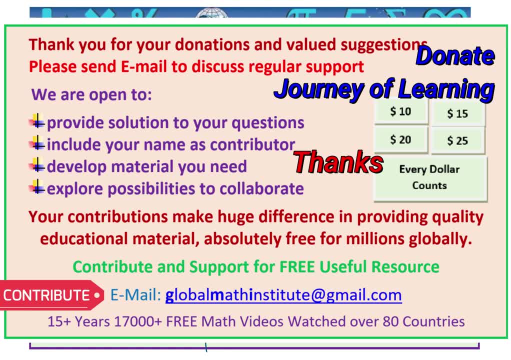 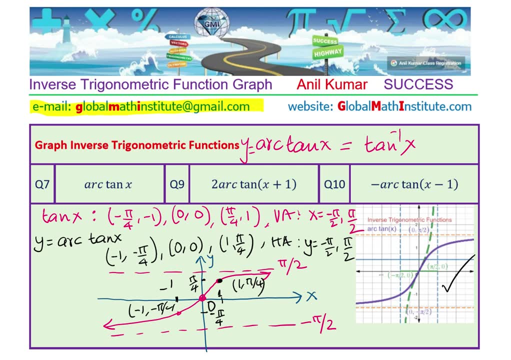 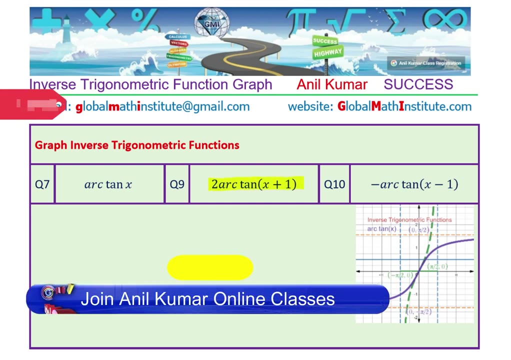 we can reach millions. so contribute for a good cause. correct, great. and also contact me on email to learn. and also, how do you join this journey of learning? okay, great. so let's now look into the transformed functions one by one. so now we'll consider two: are tan x plus one? how do we begin? 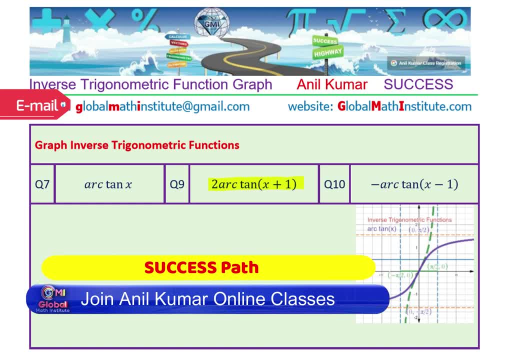 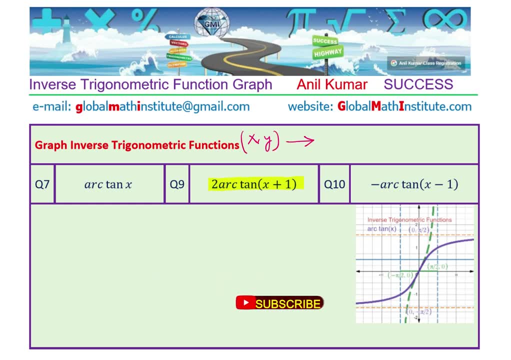 that is the first question. so first is look for the transformed points right, so the normal x, y values which were on the inverse function will get transformed. transformation here is vertical stretch by a factor of two horizontal translation one unit to the left. so the x values will be x minus one, the y values will be two times y, correct, so once again, now we'll do arc. 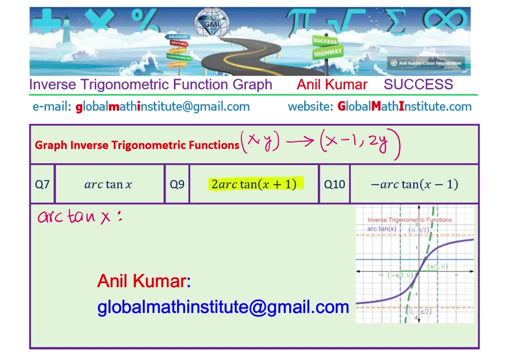 tan x right arc, tan x points which for us were, as you know, the x values now are the numbers and the y values are those radian pi by four right, and then we have correct at one. we have pi by four correct, and then we have the horizontal. 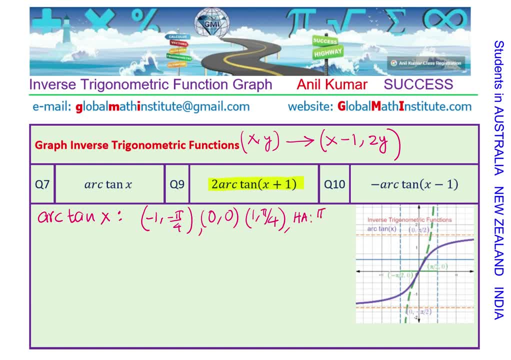 acentos correct, which are at pi by two minus pi by two. normally you'll write minus first. okay, now look into our function, which is two times arc, tan, x plus 1.. So clearly, what is happening is the y values will be doubled, but the x values minus. 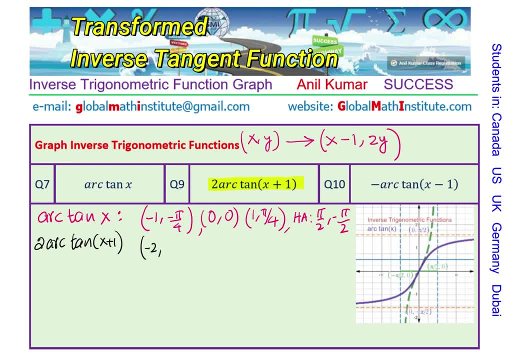 1.. So if I do minus 1,, I get minus 2.. If I double this up, I get minus pi. Make sense, right? And here minus 1,, 0, and here will be. this will come to 0 now and this will be doubled to pi by. 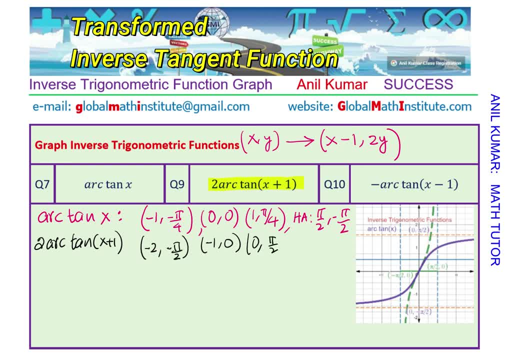 2, right- Sorry, this is pi by 2, right- And the horizontal asymptotes will now be at pi and minus pi. Make sense Plus and minus pi Clear. So that is what we are going to do. 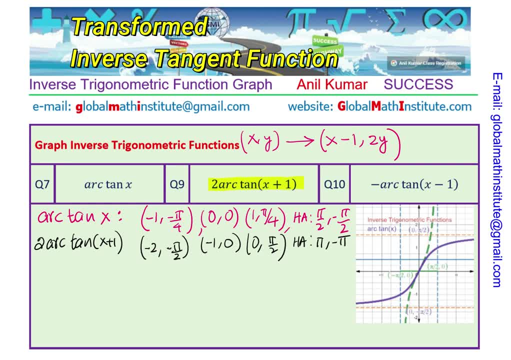 Now, if you are given this graph of arc tan x, which is shown here, practically what happens is that the horizontal asymptotes had become are twice away right. So because there is a scale problem here, I am going to sketch it on the here at this side right. 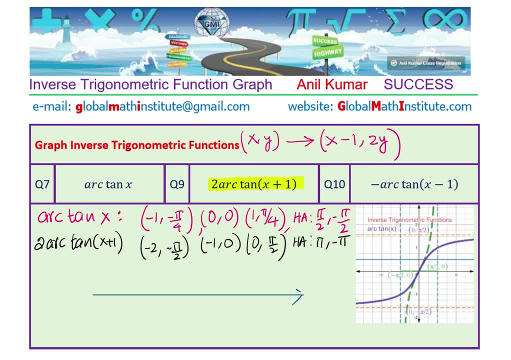 So I will do like this correct. Great, So we will assume that this is now pi by 2 for us. Is that clear to you? So this is: y equals to pi by 2, one of the horizontal asymptotes for the. 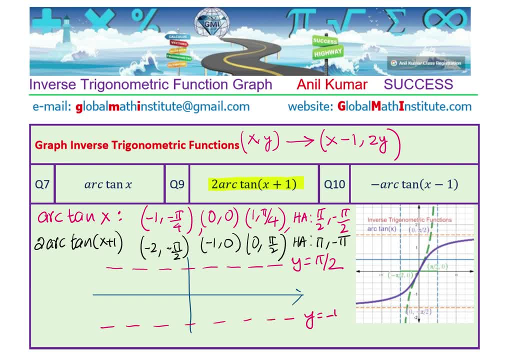 transform function. and the other one, y, equals to minus pi by 2, correct. So we are talking about 2 arc tan x plus 1. So the y values get multiplied, So pi by 2 and they become pi right. So not pi by. we multiply by 2. So y has not doubled up, So 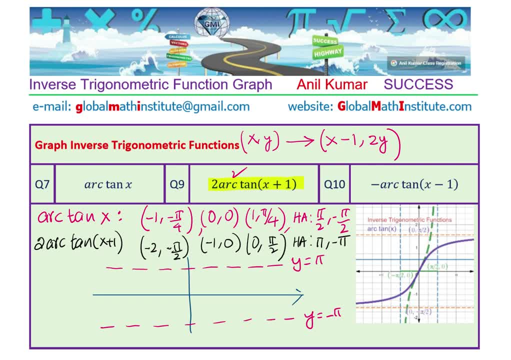 the scale is not twice, correct. So y is equal to pi and y is equal to minus pi. So those are your for tan x. Let me make it clear, right, For we are sketching 2 arc tan x plus 1, correct, The points have shifted. So so the three points. 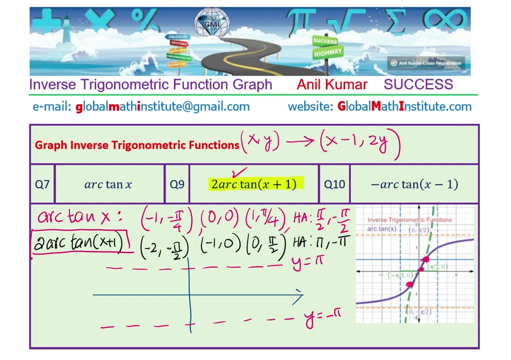 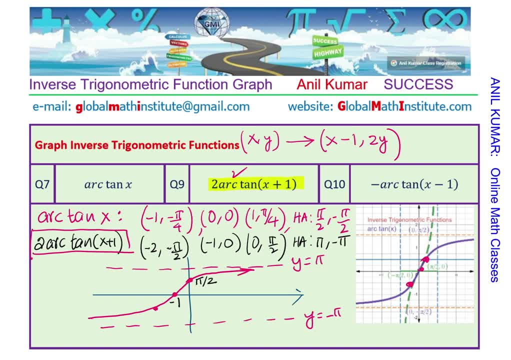 y is equal to pi by 2.. So y is equal to pi by 2.. Correct, And here we are at minus 1, and this point is at minus 2.. Is that clear to you? Minus pi by 2.. So the horizontal. 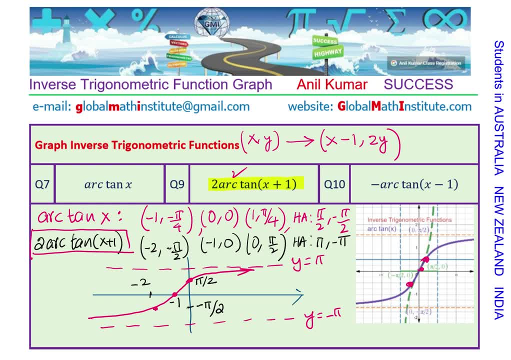 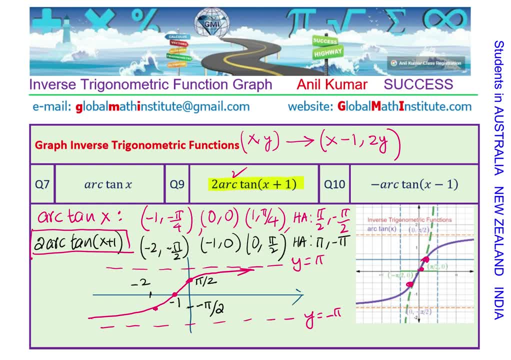 here. we have shown here. So I hope that is absolutely clear. right Now you can actually pause the video and sketch: minus arc, tan x minus 1.. Those of you who want to learn directly from me, send an email on globalmathinstitute at gmailcom. We can be part of your success story. 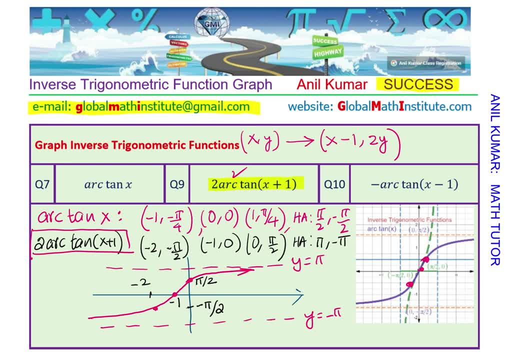 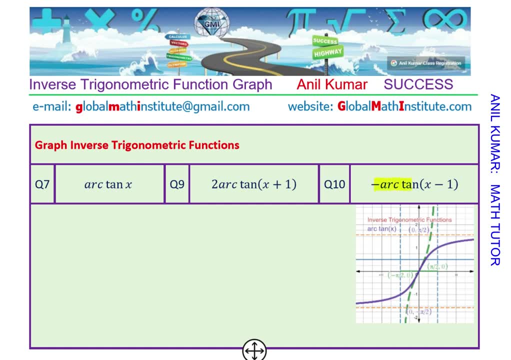 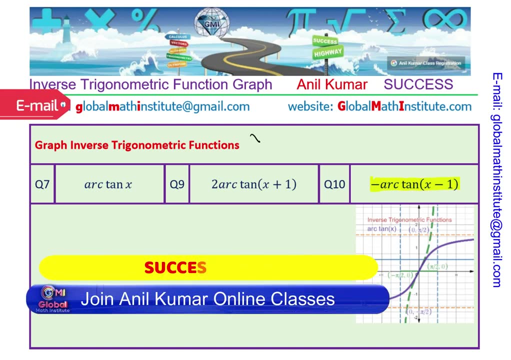 Our students get admission to the best universities and they get excellent marks. So here is the last one. So what I like you to do while sketching the graph of minus arc tan x minus 1, first thing, write the transformation. the x, y points from arc tan x will be what the x values will be added by 1 and the y values. 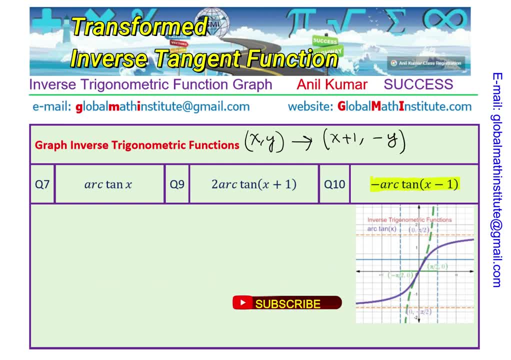 will be reflected. so minus y. so we have got two transformations here. one of them is the reflection on the x axis, the other one is translation. one unit left right, so reflection on x axis. second is translation: one unit left right, sorry, so one unit right, because minus 1. therefore x values will be this correct. 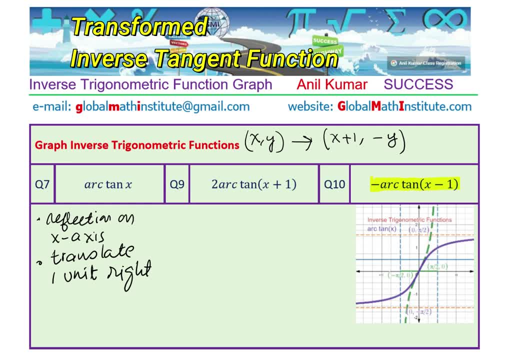 so with that, we have got the transformation of the x, y points from arc tan, x minus 1. so with that, what do we have as our good points? well, so we are always considering these three points and the horizontal asymptotes right, so the horizontal asymptote will remain same. 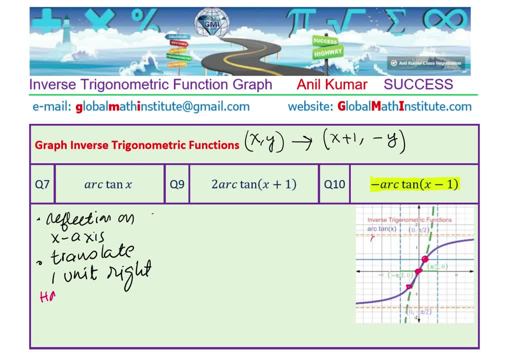 so the points will be what? so we have the horizontal asymptotes, which will remain same, which is plus, minus pi by 2, the points from left to right. the earlier point was at minus 1 minus pi by 4 will now be at 0 and reflected means pi by 4, correct? 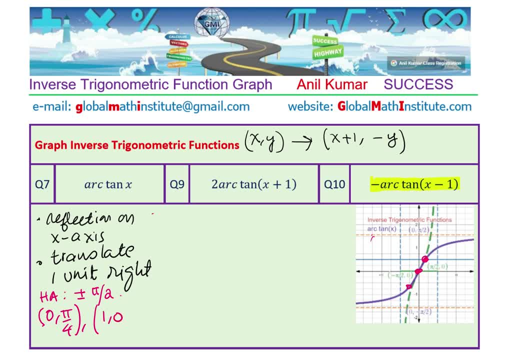 the point at origin will move one unit to the right, so 1: 0. and the third point, which was at 1 pi by 4 will be now 2 minus pi by 4. makes sense right? so we can sketch our graph on this right hand side so. 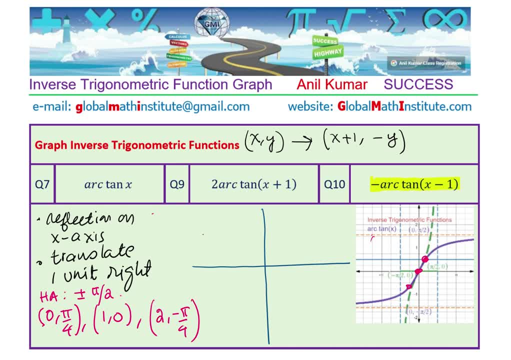 so I write that y equals to the right. so we have i equals to to the right half of points of an oblique horizontal asymptote. and one of the points to be a beer is minus pi by 2, and thus we can write: the point at origin will be at one, 4. so all this. 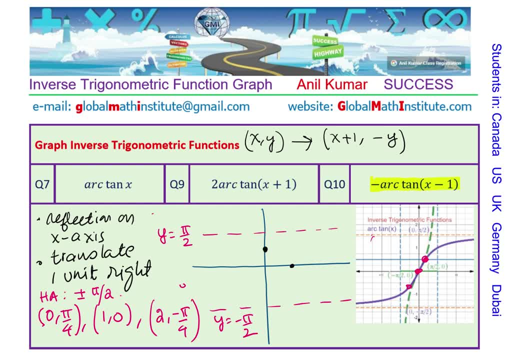 so we have a point here and then move right there and you get the idea and the whole graph will. now, since it has been reflected, it approaches always downwards, right, instead of increasing- now it is always so- it becomes always decreasing. so that is the effect of minus. you can see that the range in this case will not. 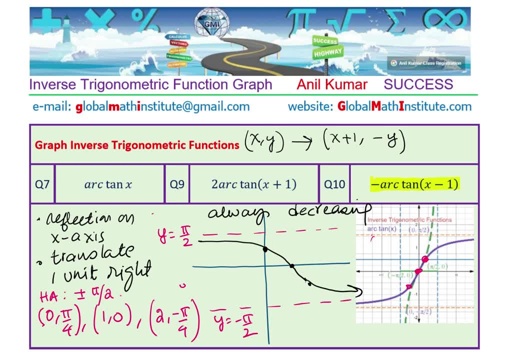 change right, so it is still the same and that is how the graph is going to be perfect. domain, of course, is from minus infinity to plus infinity. that also doesn't change with this particular transformation perfect. so I hope with this you understand how do we sketch the graph of trigonometric inverse functions.